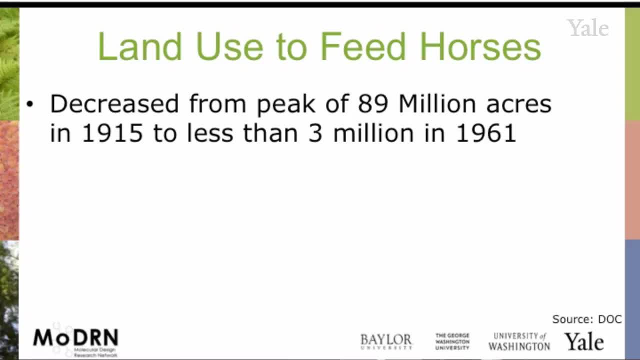 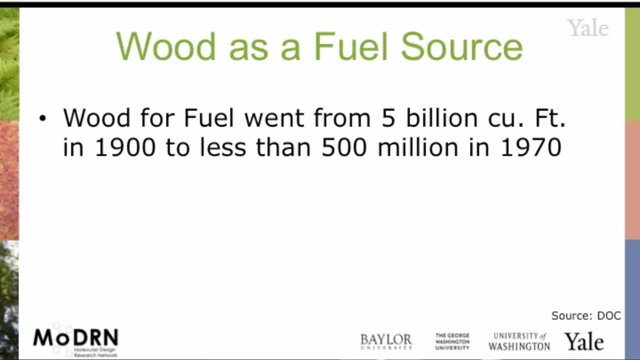 they stopped keeping the records because it was irrelevant and useless. This is the wood used as fuel. These are all from Department of Commerce. Went from a high of 5 billion cubic feet in 1900 to less than 500.. Okay, Million acres in 1970, when they stopped keeping the records because they weren't. 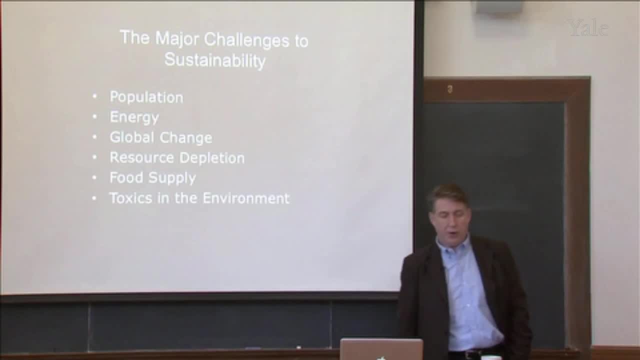 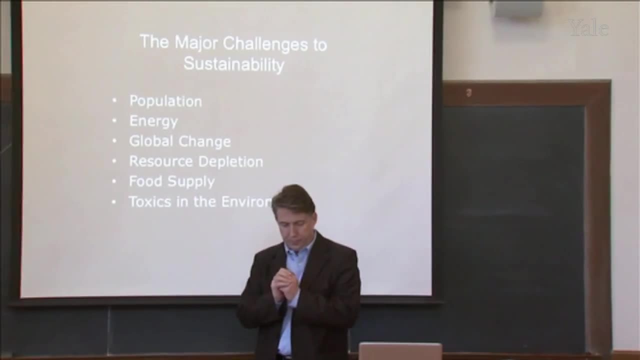 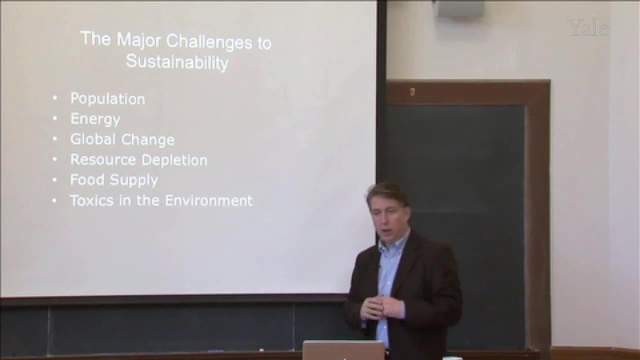 crucial to the economy. So when you there was this great New York Times article- I believe it was in 1896- that talked about the increase in horses for transportation in Manhattan And they projected the increase in population and therefore the increase in horses to transport. 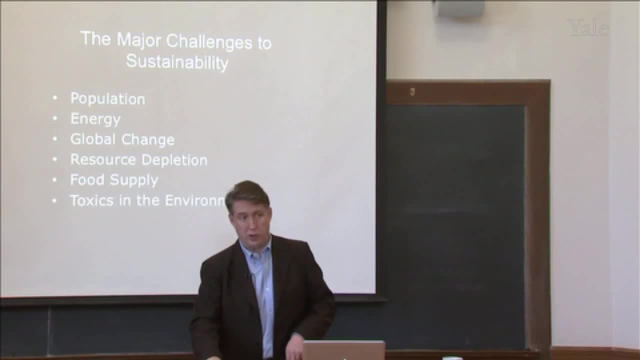 people and the increase in the natural byproduct of horses on the streets of New York, And they projected that in just a few years, the average height of that natural byproduct was going to be taller than the average person. So what happened? This was at a time when 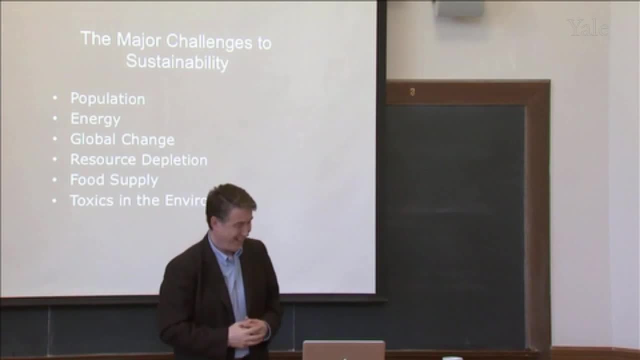 the environmental technology was a bucket and a shovel. Okay, So what happened? Did they ban horses? No Technology intervened to change the equation. It changed the trajectory we were on. You can argue about whether or not cars were the and trolley cars and. 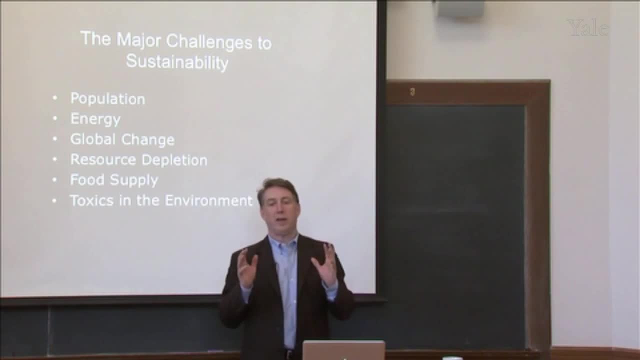 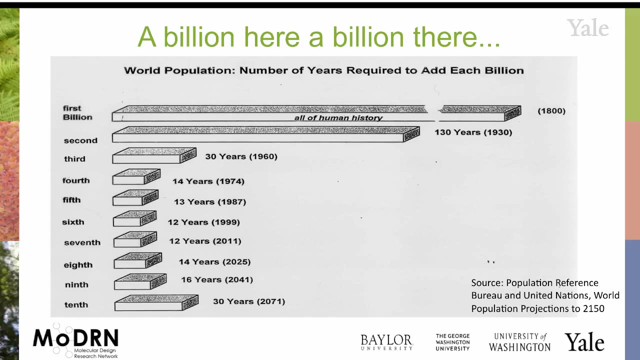 things like that were the best long-term solution, but science and technology intervened to change that unsustainable trajectory. So we start looking at the great challenges of sustainability. Everybody can have their own list, but certainly population has to be up there, right? So we're talking that. 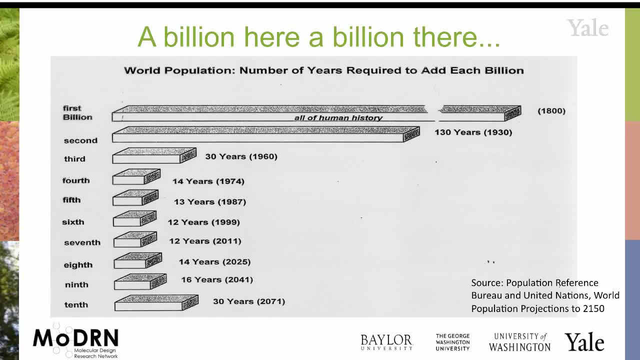 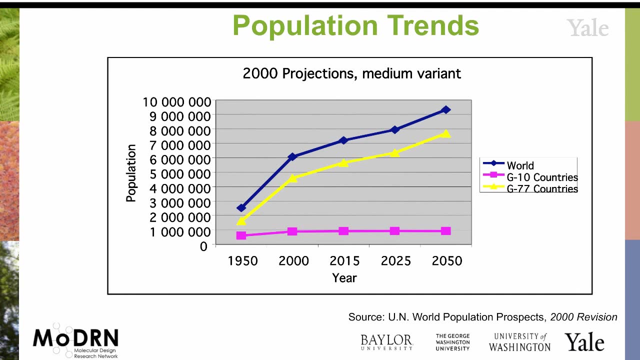 let's see, since around when I was I was born, we're more than doubled the population. We went from three billion to over seven. okay, And the past whatever 60 years? we tripled the population And where is that population growth? 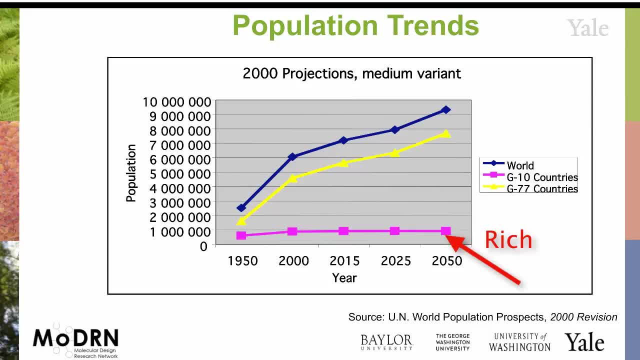 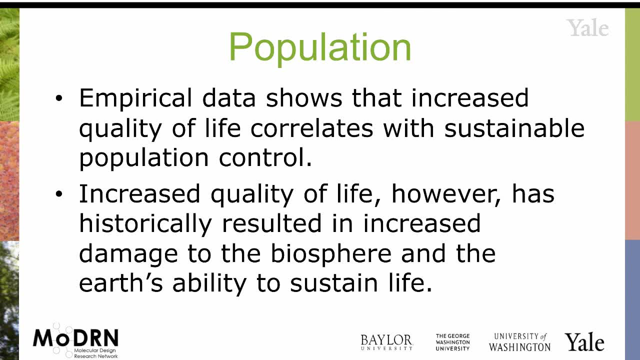 happening. These are the richest nations of the world. These are the poorest nations of the world. Okay, Great. So that tells us that what we have to do is increase the state of development of the poorest nations of the world. That will bring about higher. 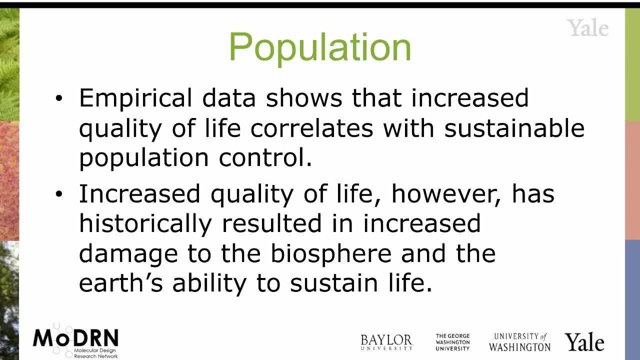 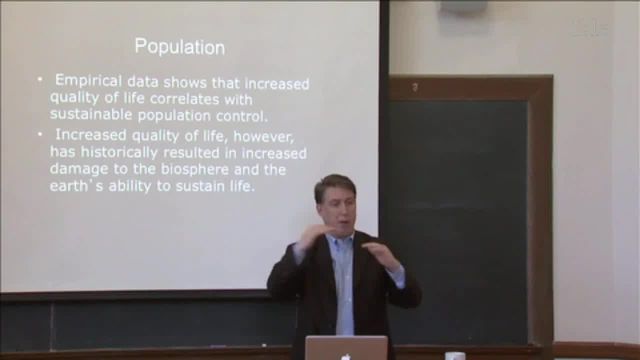 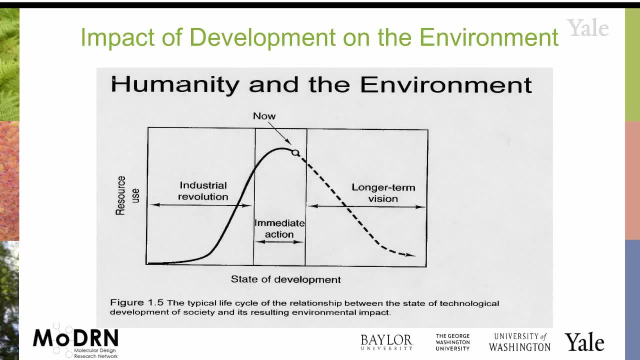 quality of life, higher state of development, higher learning follows- almost always follows higher empowerment and education of women and you bring about a stable population growth. What's the problem with that? The problem with that is that historically, coupled with increase of state of development has been increased resource depletion. 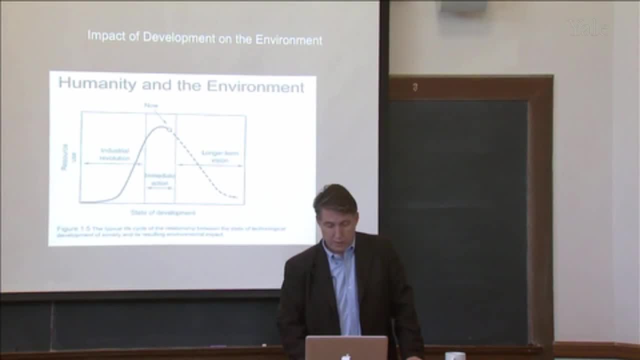 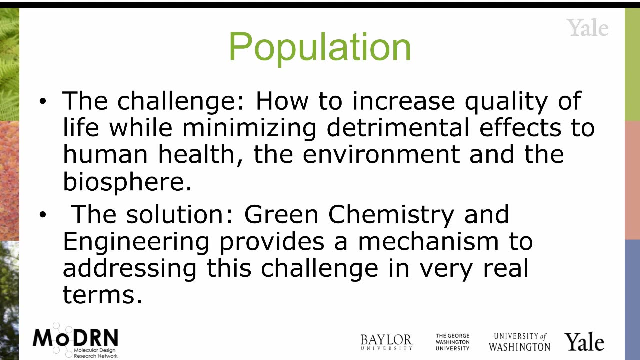 environmental degradation. All right. So the challenge becomes: how do you increase the state of development, the quality of life, while reducing the detrimental effects, the detrimental effects of this economic growth, avoiding the resource depletion? Last I checked, that's exactly what green chemistry and 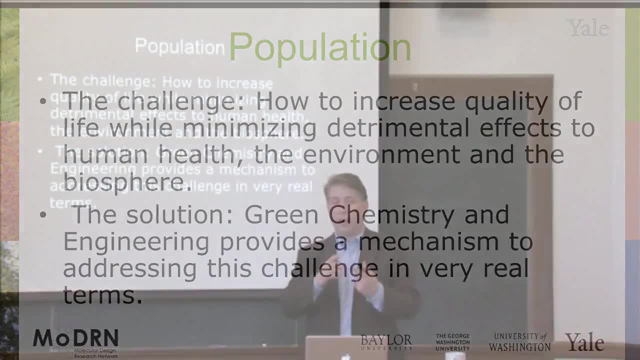 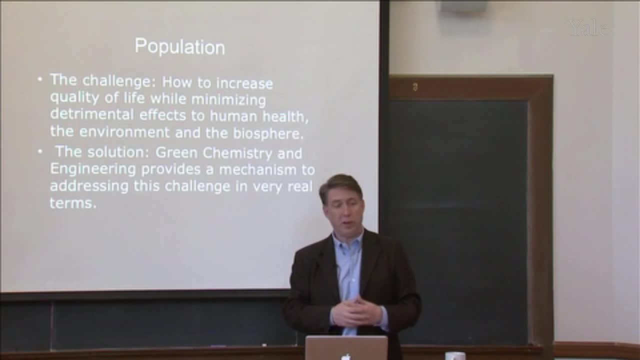 green engineering is all about How you decrease the adverse consequence, the hazard, the toxicity, the pollution, while getting higher performance. That's what we're going to be talking about this whole semester is: how do we manifest this? This is not going to be theory. We're going to be seeing countless 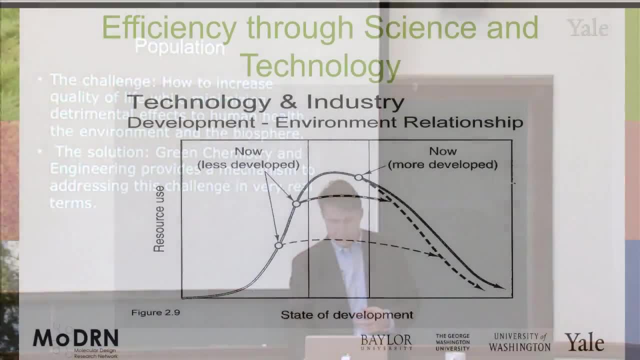 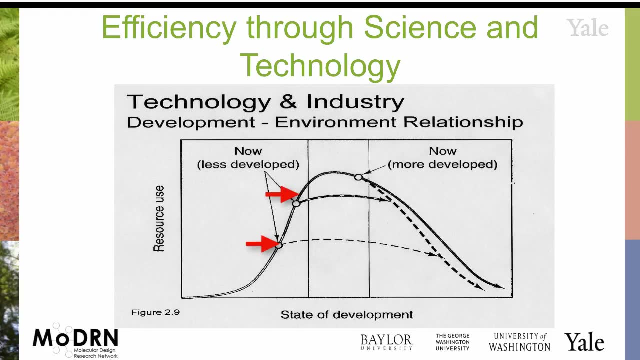 examples of how we're achieving exactly that. So what we want to do is get the higher state of development and do this kind of leapfrog technology. We're going to talk a lot about leapfrogs and I'm going to want all of you to know about. 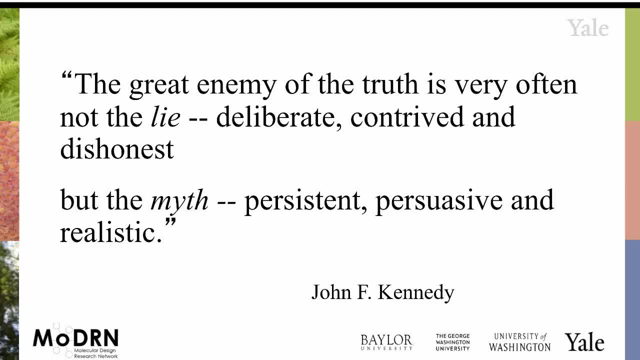 some of the leapfrog examples. Okay, This is one of my favorite of all of President Kennedy's quotes: that the great enemy of the truth is very often not the lie- deliberate, contrived and dishonest- but the myth- persistent, persuasive and 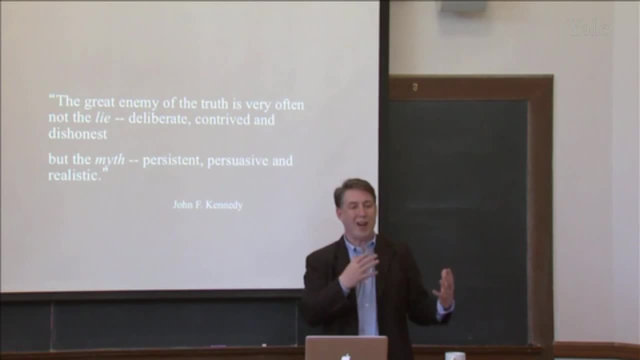 realistic. So there's a mythology that you can't have economic development, you can't have growth, you can't have increase in jobs, you can't have increased quality of life unless you're going to essentially destroy the environment, use toxic substances. Green chemistry is belying that myth every day. 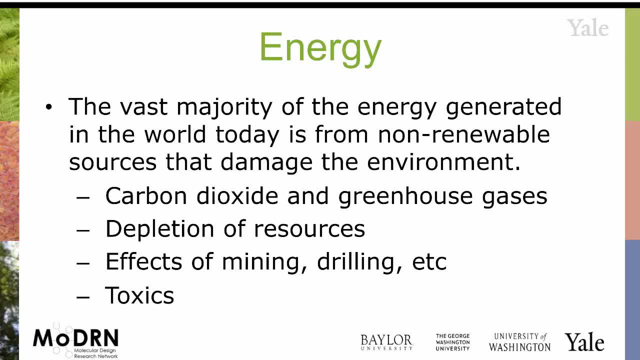 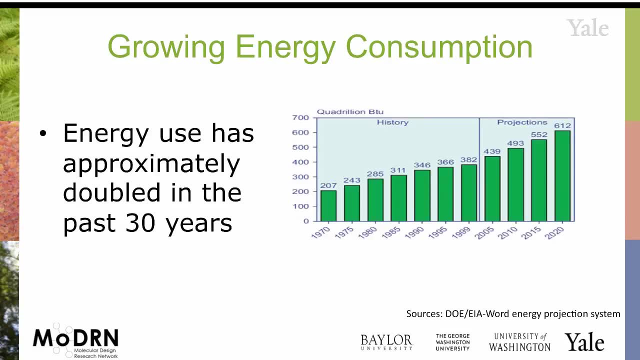 I'm going to talk to you a little bit about some of these. So let's talk about energy. Everybody knows, and this room knows, that the vast majority of our energy in the world today is generated from non-renewable sources. All right, I'm going to talk a little bit about energy. Everybody knows, and this room knows, that the vast majority of our energy in the world today is generated from non-renewable sources. All right, 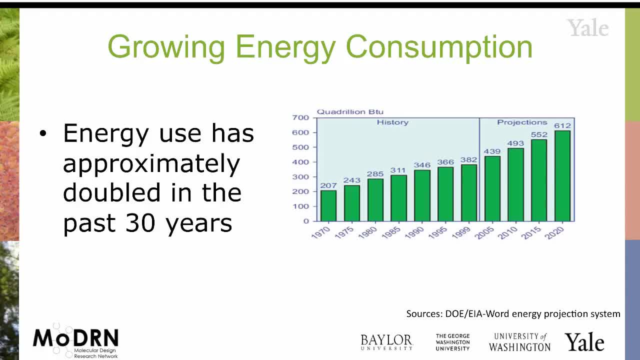 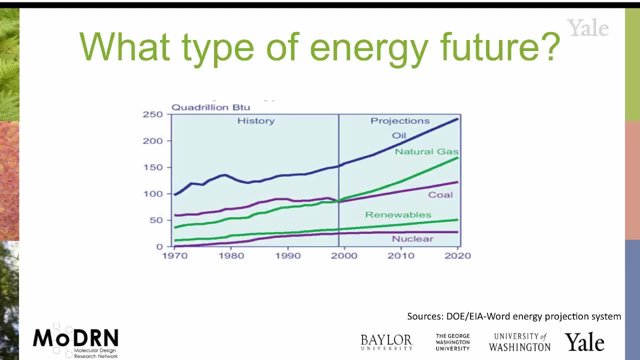 So this is the projected increase in consumption of energy over time. These are the projections And this is what is projected to be the portfolio of energy: Still oil, still natural gas, still coal. What green chemistry, green engineering, sustainable design is all about is changing that trajectory, changing that. 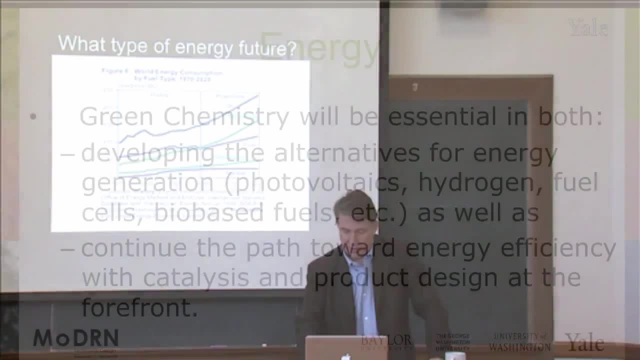 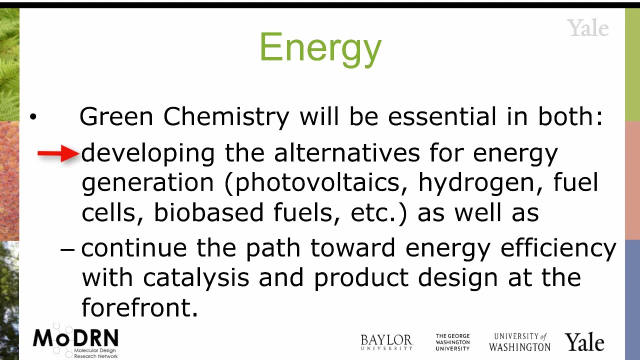 balance, so that, though, that is not inevitable, All right. So it's looking at developing alternatives for energy generation, Everything from photovoltaics, hydrogen generation, fuel cells, bio-based- In addition to these alternative energy sources that we're going to talk a lot about, it's also about 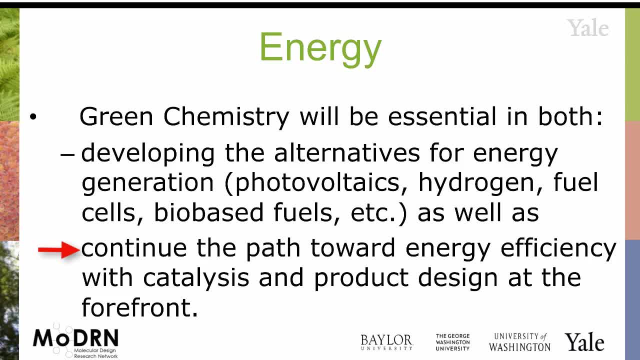 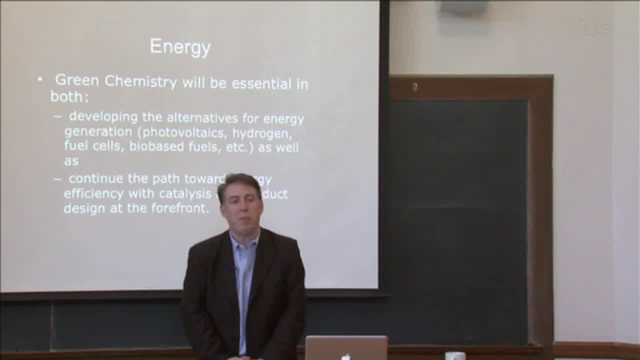 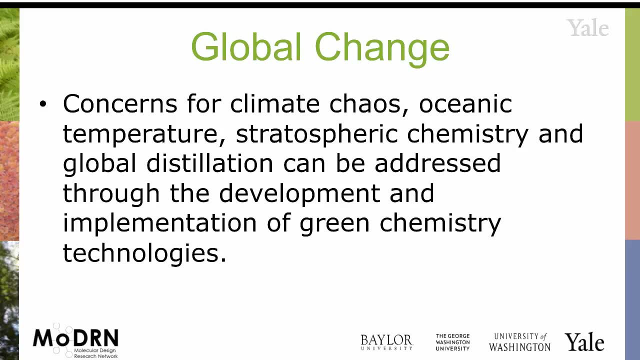 catalysis. We're going to talk about catalysis and how you can undertake transformations, for instance, of one material into another, with dramatically lower energy, with dramatically lower waste, with dramatically lower material consumption. Global change- All right. I hate the phrase global warming. I. 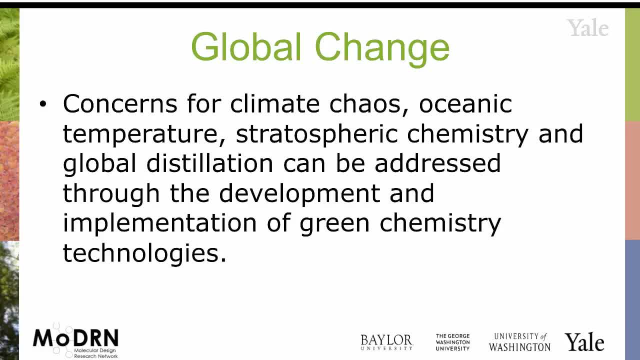 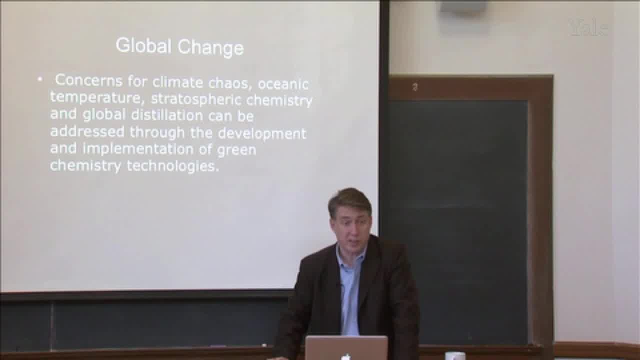 sometimes use the phrase climatic chaos, because what's happening is we're adding energy into what's largely a closed system, And when you do that, some places will get warmer, some places will get colder, some places will get wetter, some places will get drier. It's not about this. 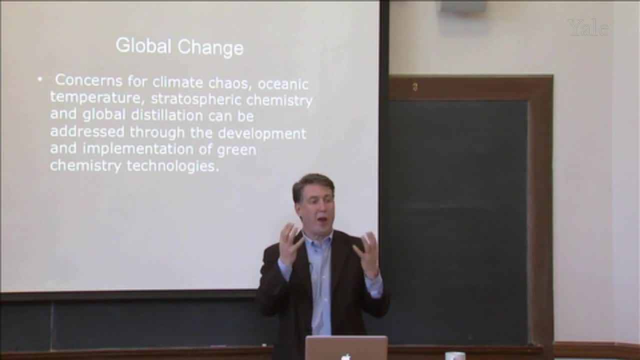 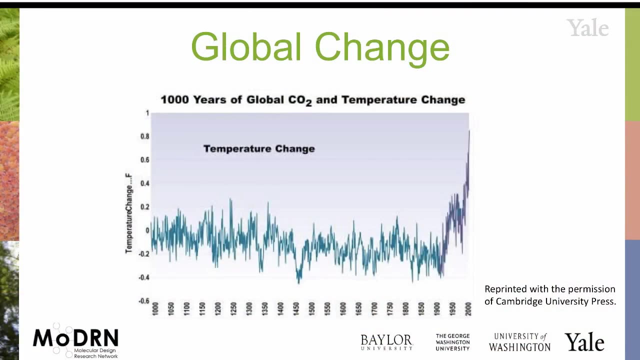 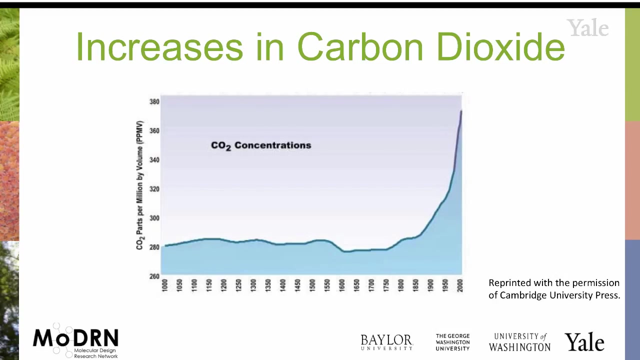 this linear progression. It's about how you add turbulence into into a system and the literal definition of the word chaos. This is one of the classic pieces of data. This shows the temperature change over the past thousand years. This shows the increases in carbon dioxide concentrations over the last several. 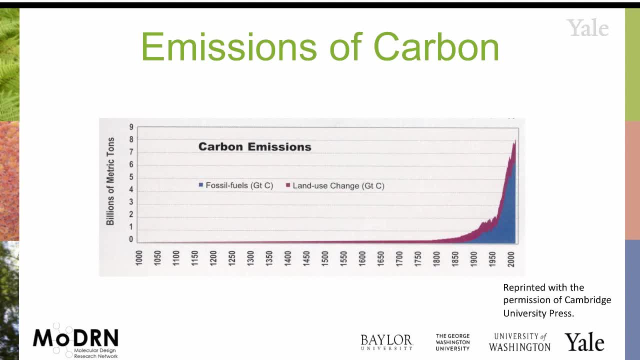 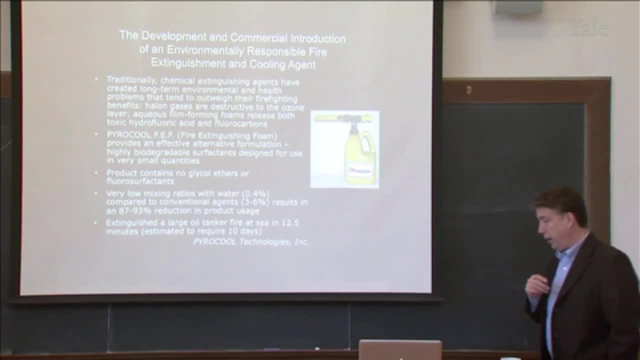 years. And these are the emissions over time. Okay, All right, So I'm telling you this quick story. One of the most powerful greenhouse gases is not is not CO2, but a lot of the CFCs, the chlorofluorocarbons And 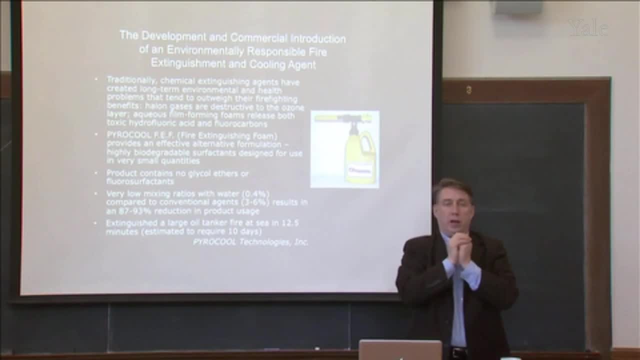 many of these were were used as fire extinguishing agents. Okay, This is an example of a technology- it's called Pyracol, of a fire extinguishing agent, And this is a technology that that didn't use CFCs- completely eliminated CFCs And so no. 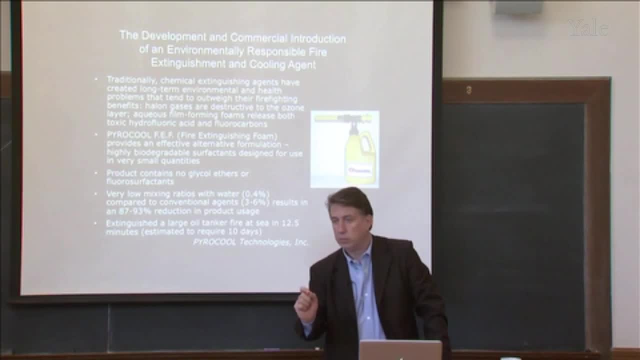 emissions. It basically served to make water a more effective fire extinguishing agent by using surfactants in a in a formulation Okay. So why do I tell you that? Because CFCs are such a big deal in fire extinguishing agents and they contribute even though they're. 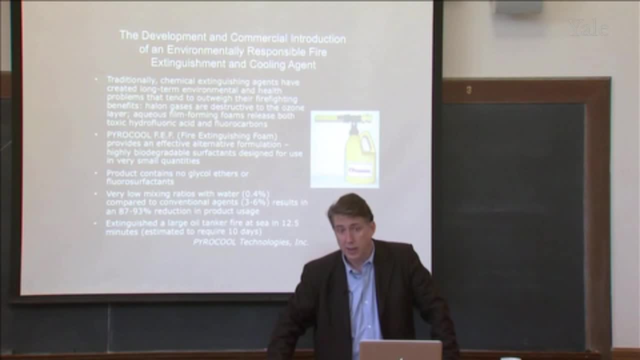 about 24,000 times more potent a greenhouse gas than CO2.. No, that's not why I'm telling you that. I'm telling you this because one you can use the science and technology of this technology to use in other applications. 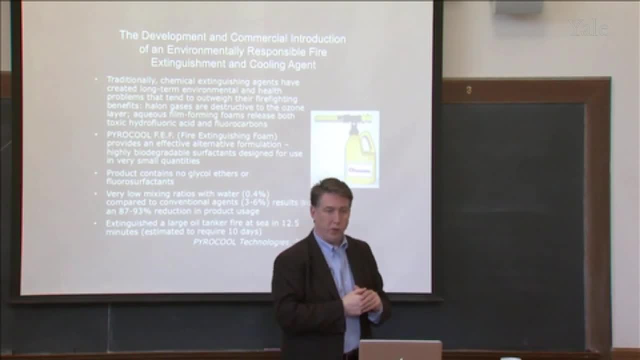 But, more importantly, when this fire extinguishing agent was used in an oil tanker fire in the Bosphorus Straits, Lloyds of London estimated that this would take 10 days to put out, and this fire extinguishing agent put it out in 12 and a half minutes. 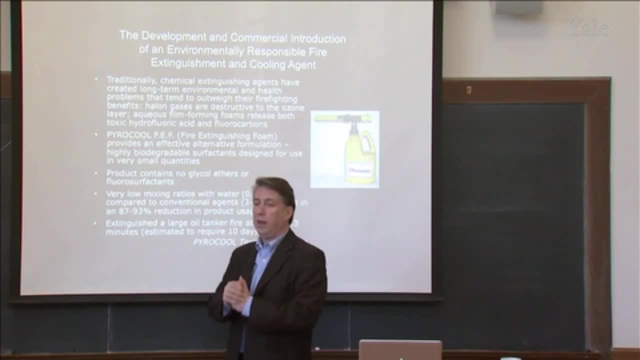 So what does that mean? Come back to JFK: The great enemy of the truth is very often not the lie, It's the myth. The myth is that green products are not going to work as well, that if you're going to get environmental benefit, if you're not going to have environmental degradation, you're. 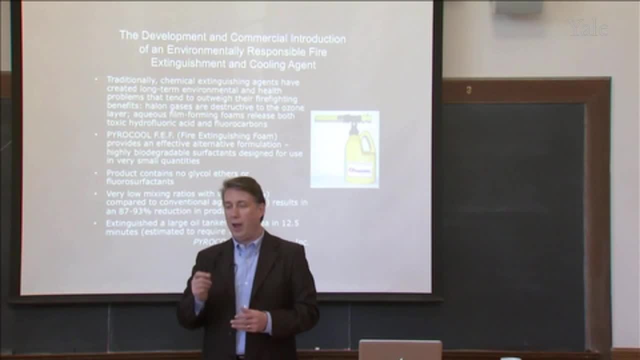 not going to get the performance and the function that you want. I am going to show you. you're going to discover. you're going to research examples over and over again, Thank you- That are more functional, higher performance and environmentally beneficial and sustainable. 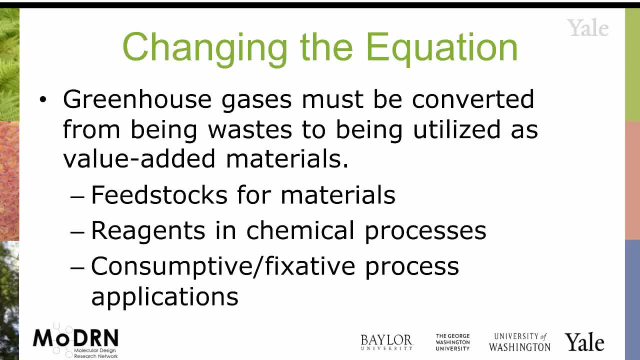 So how do we change the equation? It's not about just CFCs or the like. How do we make greenhouse gases so that they're actually functional? How do we take CO2 and build it into our polymers and plastics? It's being done. 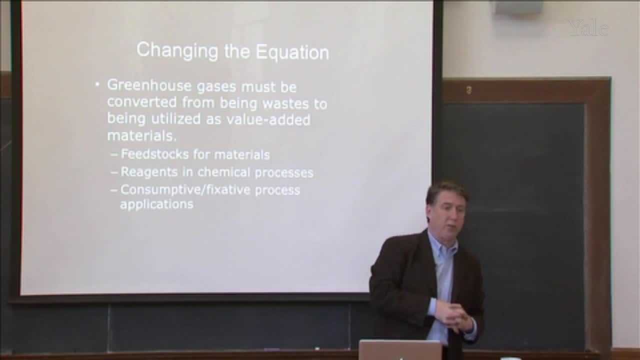 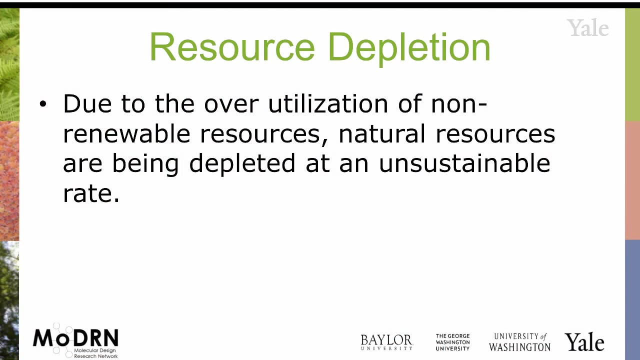 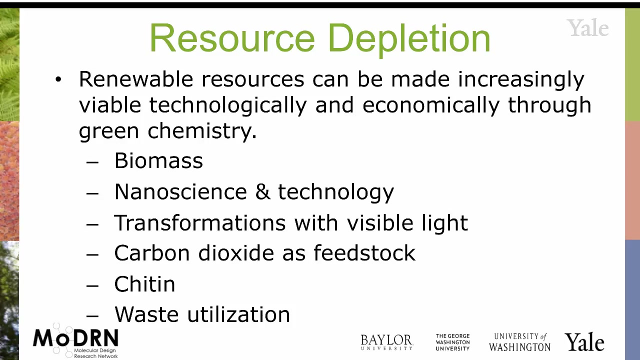 Brilliant work by a company founded by Professor Jeff Coats and Cornell making new plastics using CO2.. All right, So we know that we have a resource depletion issue that we've talked about, that We know that we're burning a lot of our natural capital like it's a fire sale. 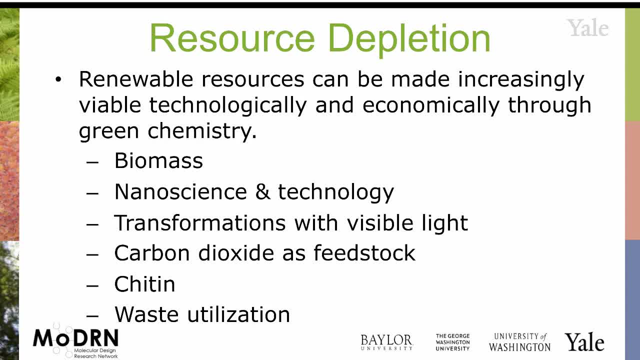 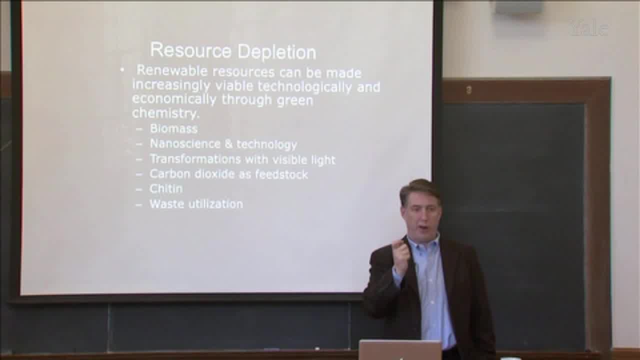 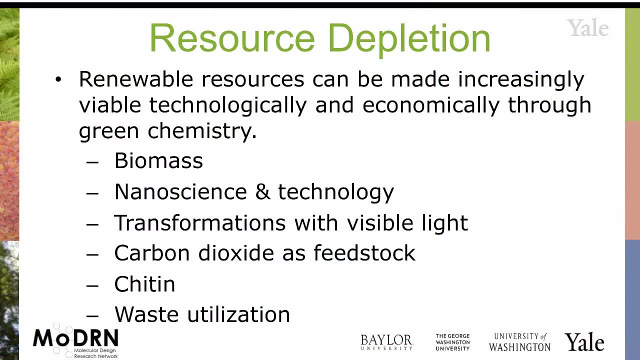 How do we what green chemistry is doing is, how do we use biomass, How do we use nanoscience so that we get the function that we want, That we want with dramatically less material? How do we go to carry out transformations with visible light rather than chemicals and 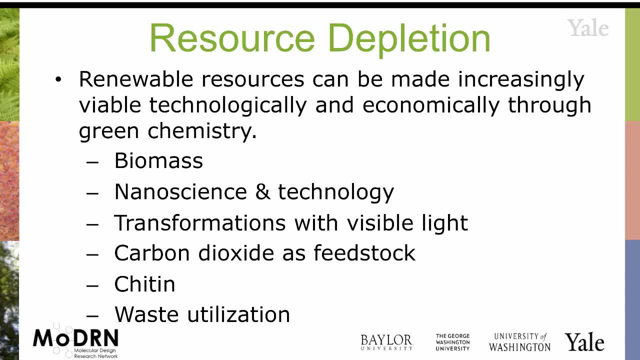 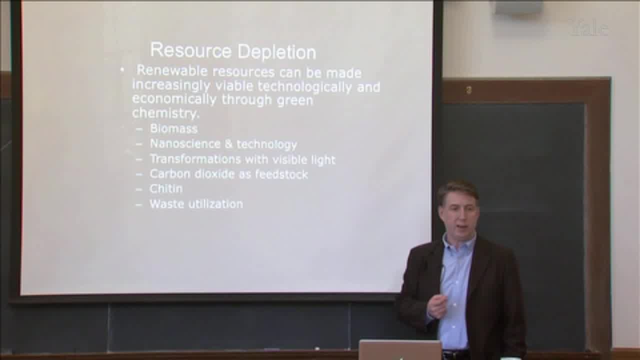 material. How do we use carbon dioxide as a feedstock rather than as a waste? Remember when is a waste not a waste when it's a value-added material. All a waste is is a material or energy for which you have not found a valuable endpoint. 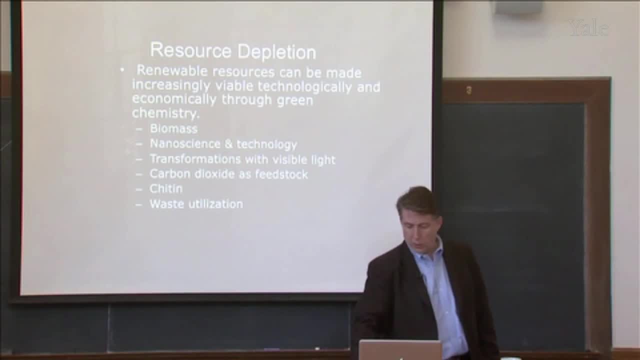 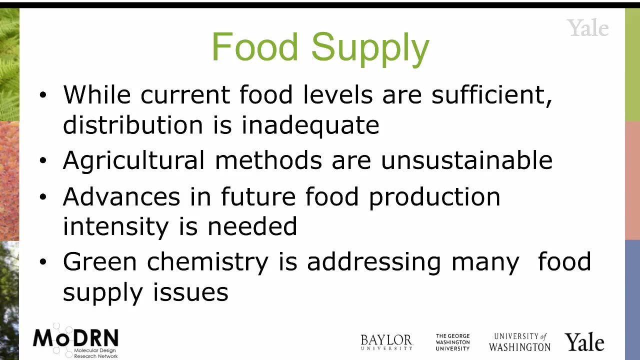 And carbon dioxide. Carbon dioxide is a biopolymer or a waste utilization. All right, I'm going to be wrapping up talking about food supply. We actually produce enough food. There's inequitable distribution, so there's still regional starvation, which is tragic. 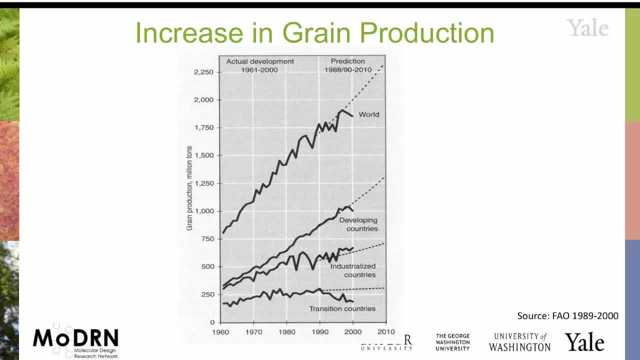 But if you take a look at the Green Revolution that I talked about with Norm Borlaug, this is the development since 1960 of food production: Absolutely astounding Food production in developing countries and industrialized nations- both you have to ask the question: how did it happen? 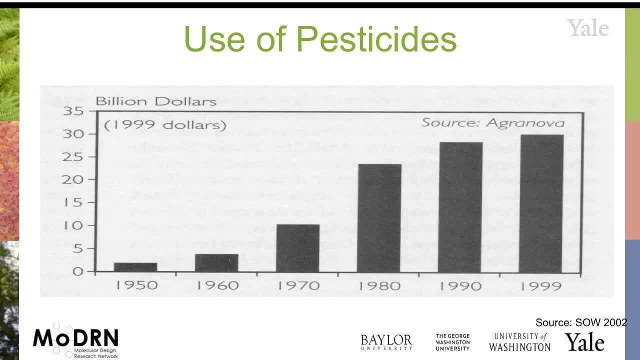 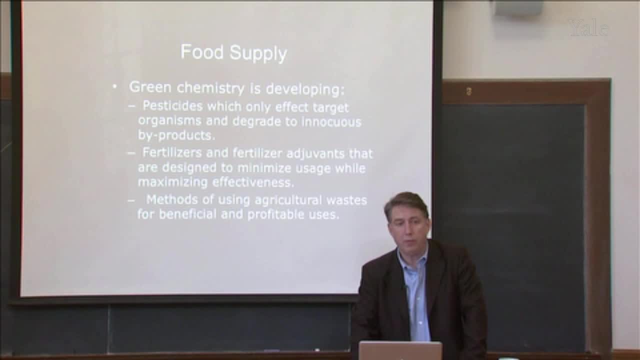 That's part of how it happened. That's part of how it happened. So how do we get that important performance- producing food, feeding hungry bellies, but not doing it in a way that's contaminating our drinking water- building up in our bodies? 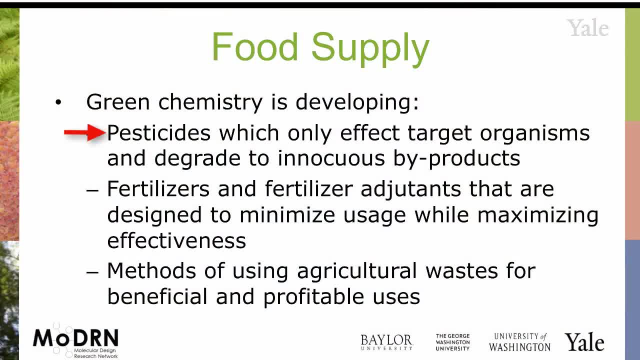 and that's what green chemistry is: developing New pesticides which are only focused on the target pest and not all of the other beneficial insects. Fertilizer and fertilizer adjuvants that draw the fertilizers to the roots so that you don't. 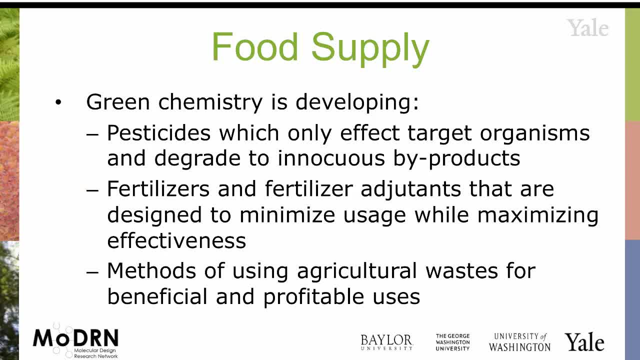 put ten times the amount of fertilizer so that you wind up having it get into your drinking water, but you only put down what is actually going to be taken up by the plant. Methods of using agricultural wastes for beneficial and profitable use. All right.